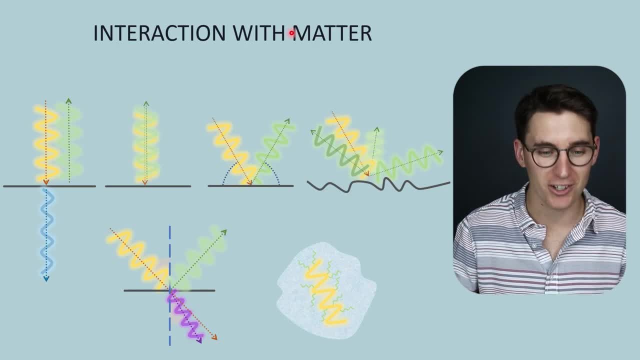 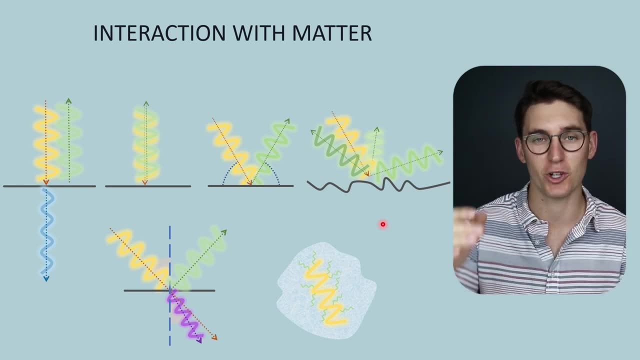 known as acoustic impedance. Now, when we look at ultrasound interactions with matter, you can see there are multiple different types of interactions, And all of these we are going to cover in the following two talks. Now, in this top row here, this is what's called reflection, where we have 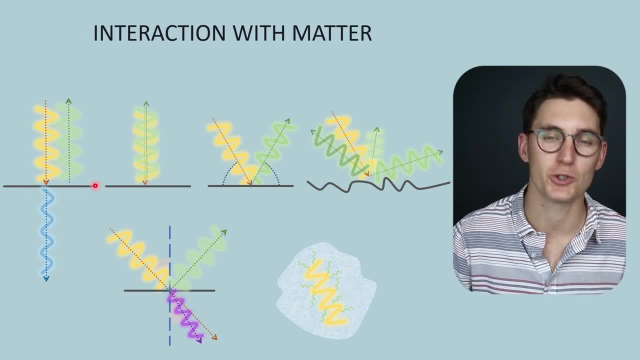 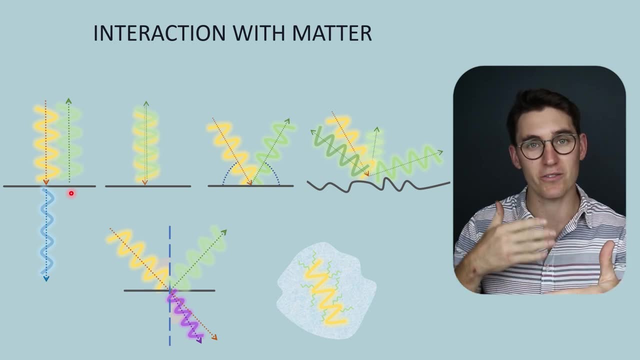 an incident ultrasound wave reflecting off a tissue boundary. Now, a tissue boundary describes the interface between two separate tissues. We can have ultrasound wave going through muscle and then going through fat. That boundary between the muscle and the fat is what's known as a tissue boundary And that's commonly 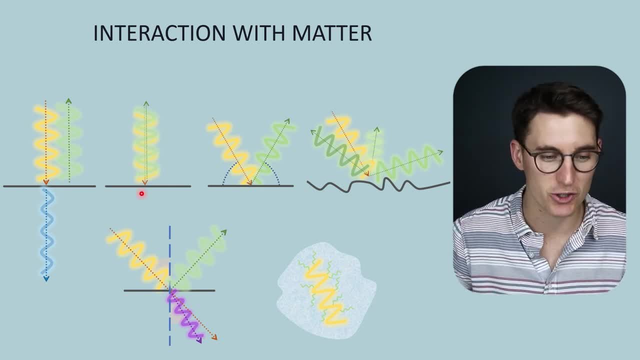 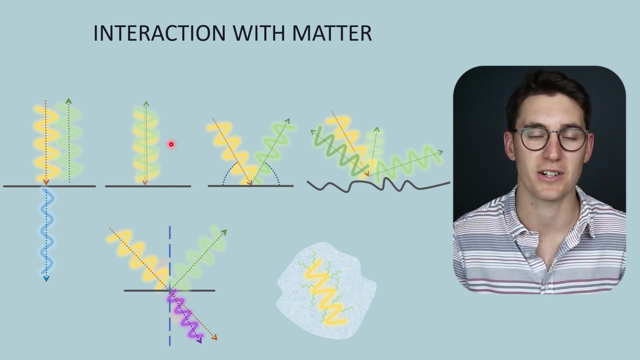 where tissue interactions occur. Now, at these tissue boundaries, we can get reflection, either partial reflection of that wave, with some of that incident wave being transmitted through to the next tissue. complete reflection of that incident wave where all of that energy returns as an echo towards our ultrasound machine. 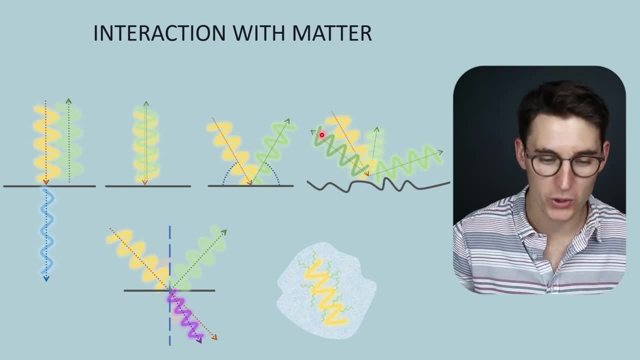 what's known as specular and non-specular reflection, both of which we'll look at in our next talk. Then, if an ultrasound wave interacts with a tissue boundary at an angle and the speed of sound between these two different tissues varies, we get what's known as refraction, And 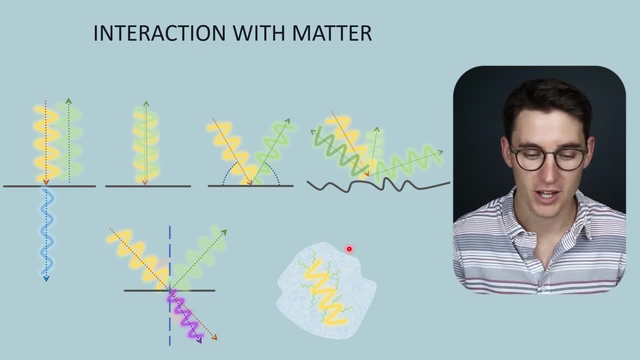 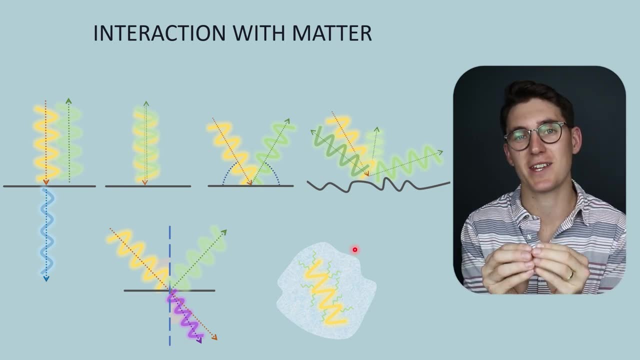 we're going to spend an entire talk looking at refraction itself. The last type of tissue interaction we get is what is known as scattering Now, when an ultrasound wave interacts with units within that tissue that are smaller than the wavelength of that incident ultrasound wave. 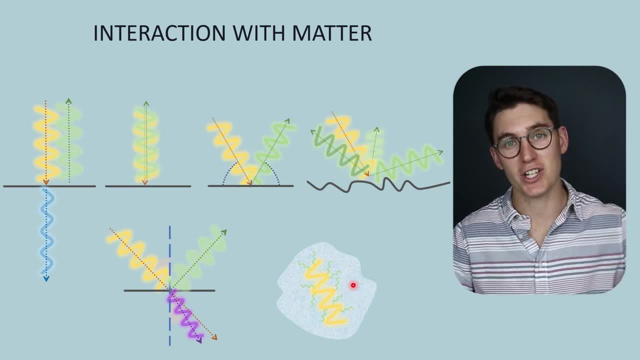 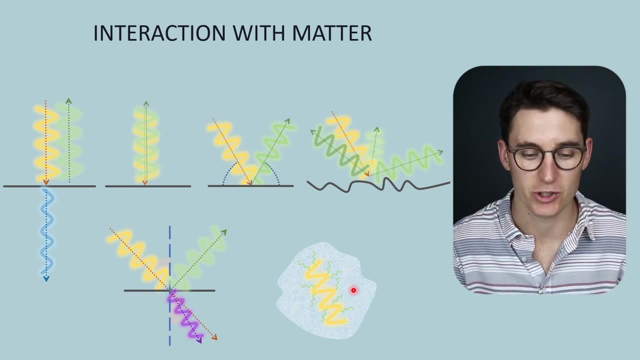 we get what's known as scattering. We get loss of energy of that incident, ultrasound wave with small sound waves being produced in any direction, scattering out amongst the tissue. Now I like to think of scattering as a large wave in the sea coming towards a beach that is made of pebbles. 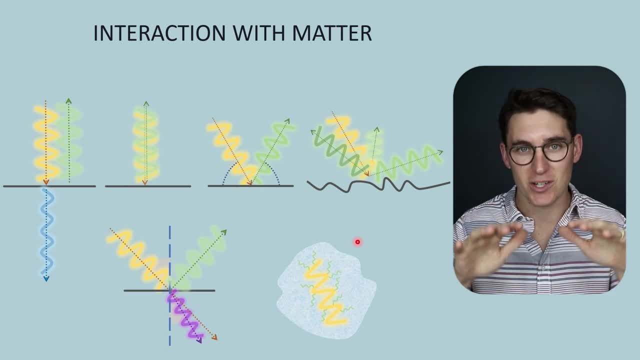 Now, those pebbles are much smaller than the wavelength of that wave and as that wave crashes into the bank, that wave disperses in all directions As it interacts with those pebbles, and that's what we get with scattering: the energy is dissipated. 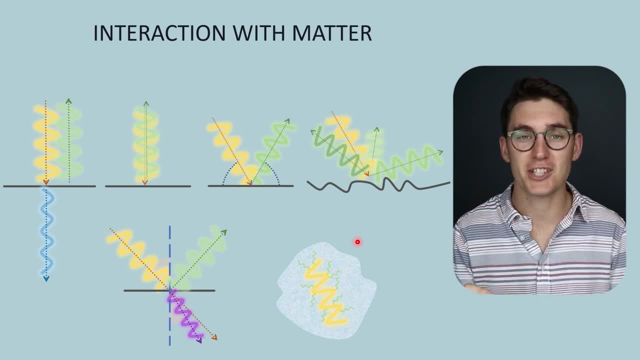 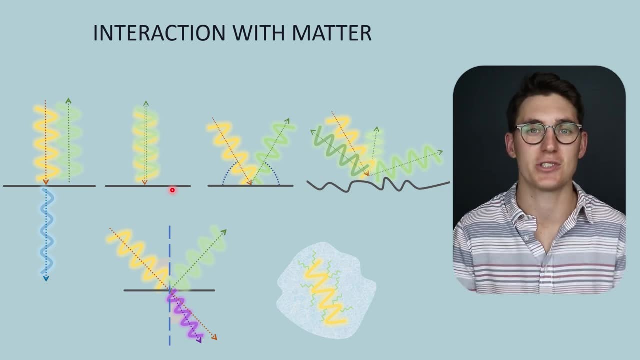 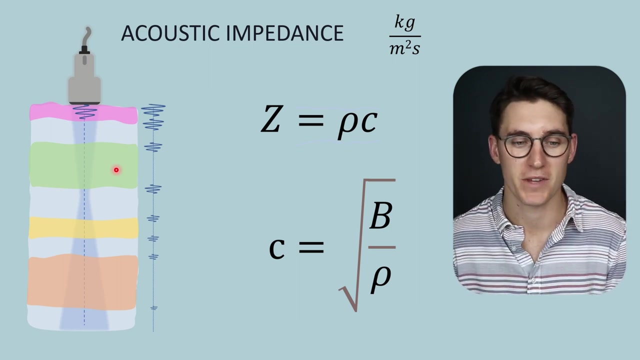 out into lots of smaller little waves. Now I've mentioned that it's acoustic impedance that determines these interactions at tissue boundaries. So what exactly is acoustic impedance? Well, acoustic impedance is an inherent property that is specific to a specific tissue type, And we denote acoustic 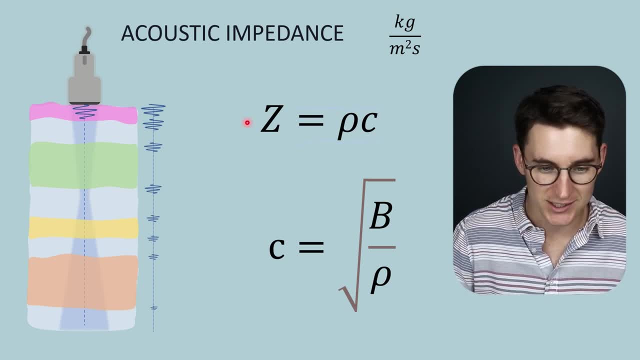 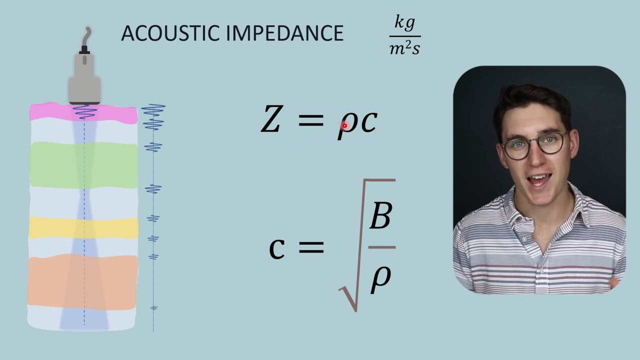 impedance by the letter Z, here this capital Z. This is acoustic impedance, And acoustic impedance is calculated by the product of both the tissue density and the speed at which sound travels through that tissue. Now we measure density as kilograms per meter cubed. how much weight is there? 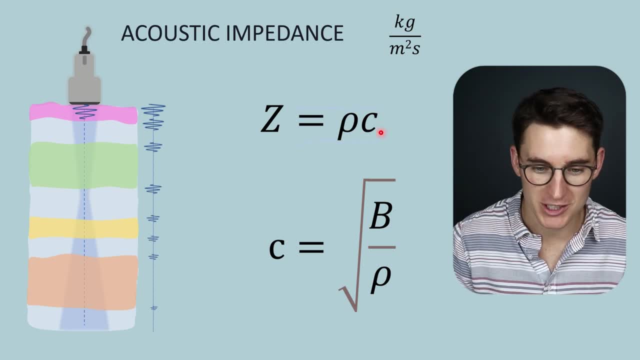 within a cubic meter of tissue And we've determined speed as meters per second. So our acoustic impedance SI units are kilograms per meter squared per second. Now, as you can see, the tissue density, as well as the speed, contributes to this acoustic impedance. 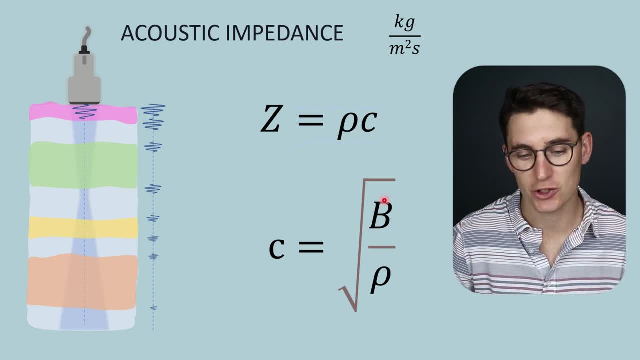 And we've seen that speed is determined by the tissue's bulk modulus, its stiffness, its resistance to compression and the tissue's density itself. And because we're multiplying density by speed, here we can see that it's the bulk modulus itself that contributes the most to acoustic. 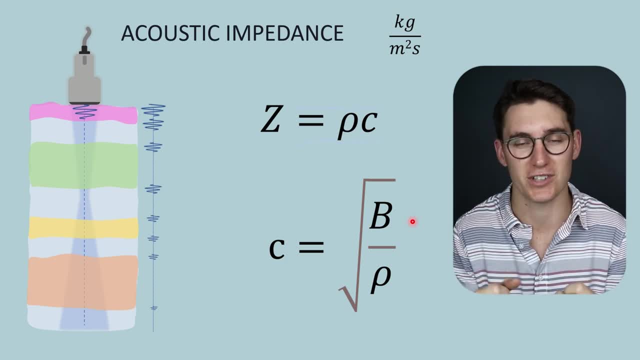 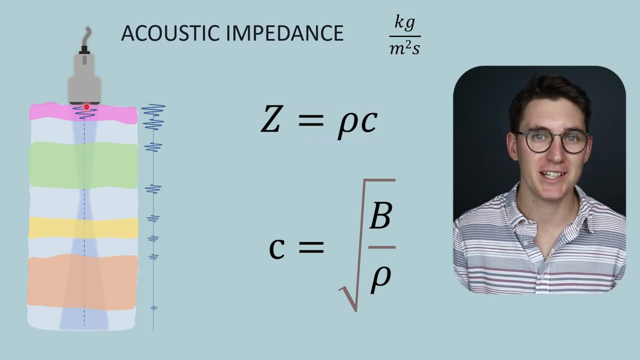 impedance. So it's the tissue stiffness or lack of stiffness, the tissue's compressibility or resistance to compressibility that determines the acoustic impedance. So when we release an ultrasound pulse into a patient's tissue and that pulse comes into contact with a 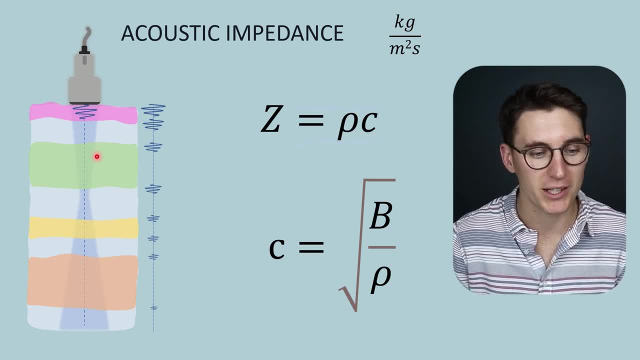 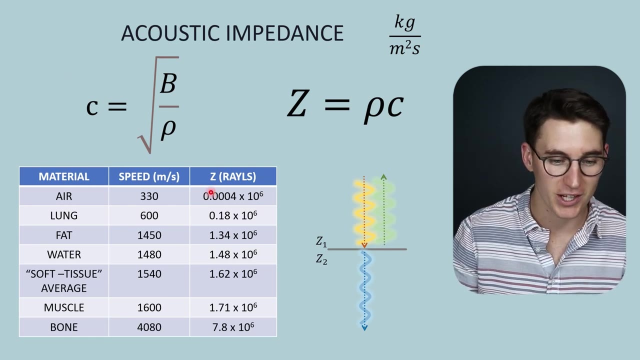 tissue boundary. here it's the difference in acoustic impedance between those two tissues that will determine how much of that ultrasound wave is transmitted through that tissue boundary and how much is reflected back as an echo towards our ultrasound machine. So here I've tabulated the various different acoustic impedance values for different soft tissues that we 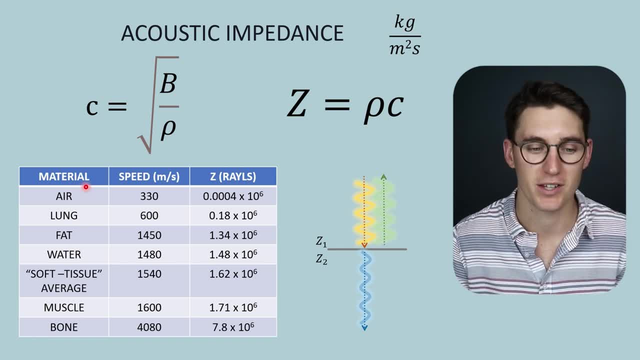 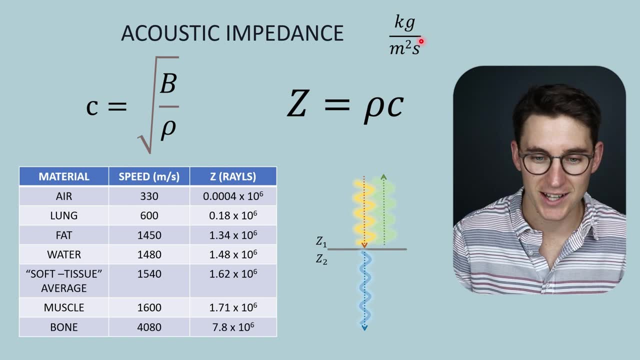 may come into contact in diagnostic ultrasound imaging. Now the acoustic impedance SI units we've seen here are kilograms per meter squared. second, Now there's another special name given to this, which is known as rails, and this is the value we generally use when talking about acoustic impedance. Now we can see the rail value between air and bone. 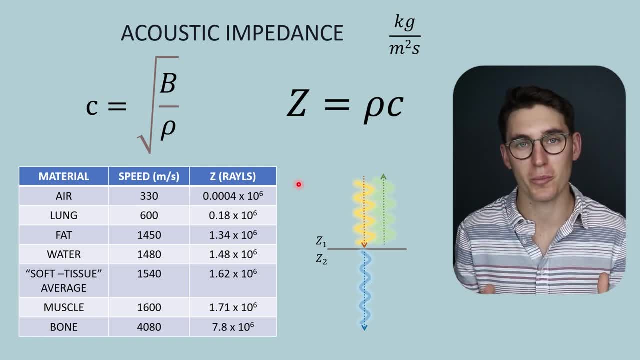 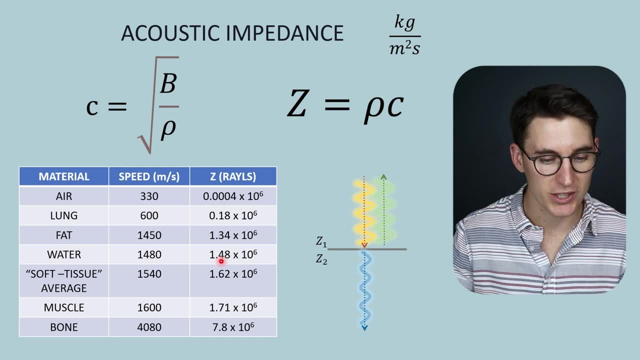 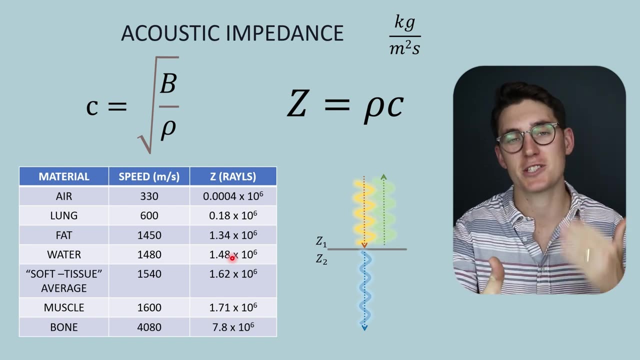 There is a vast difference here, and that's the bulk modulus predominantly that accounts for this drastic change in acoustic impedance values. Now, if the two tissues have similar acoustic impedance values, most of that ultrasound wave at that tissue boundary will be transmitted with a very 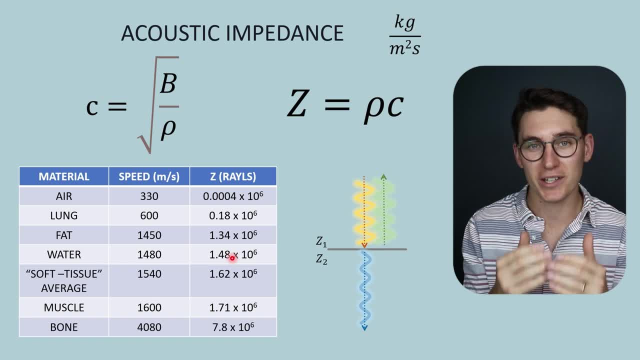 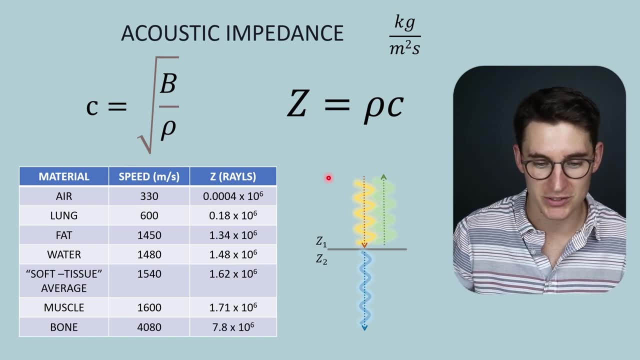 small echo coming back And in our next talk we're going to look at how we can calculate the transmittance value versus the reflected ultrasound value. Now, when we look at a tissue boundary, we've seen this diagram. now at the beginning of the talk we talk about the acoustic impedance. 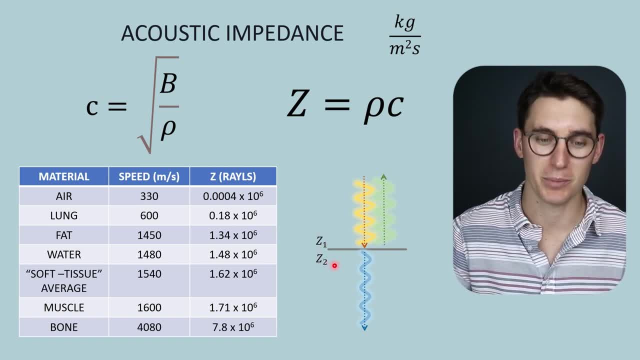 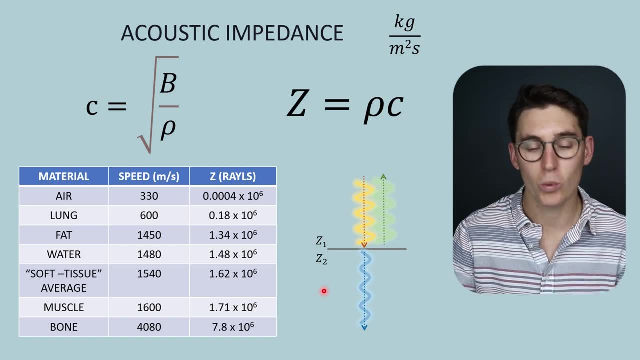 value of our first tissue and compare that to the acoustic impedance value of our second tissue. here Now, when there is a large difference in these two acoustic impedance value, we will get most of that ultrasound wave reflecting back towards our ultrasound machine. Now it doesn't matter if the difference is coming from a low acoustic impedance to a high acoustic. 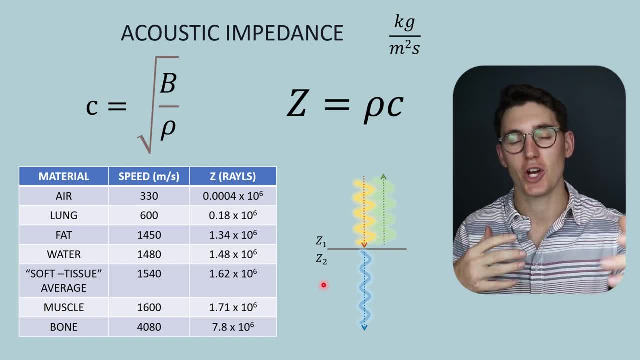 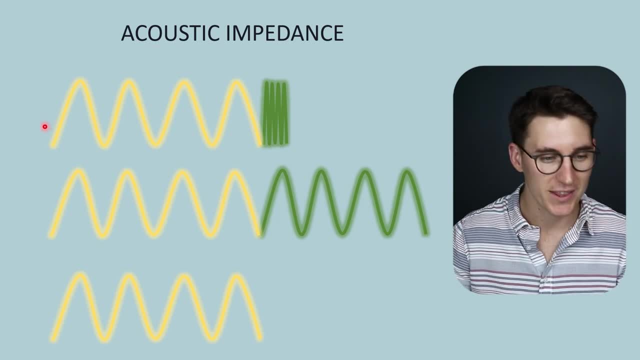 impedance or vice versa. As long as that difference is large, we will get a large reflection back. The best way to think of this is think of this yellow wave as our incident ultrasound wave. This is coming through our first tissue and interacting with our second tissue here. 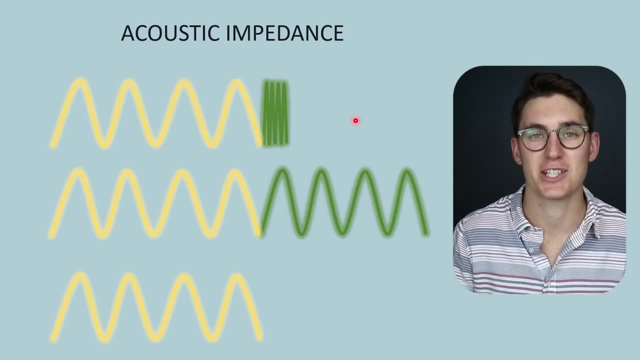 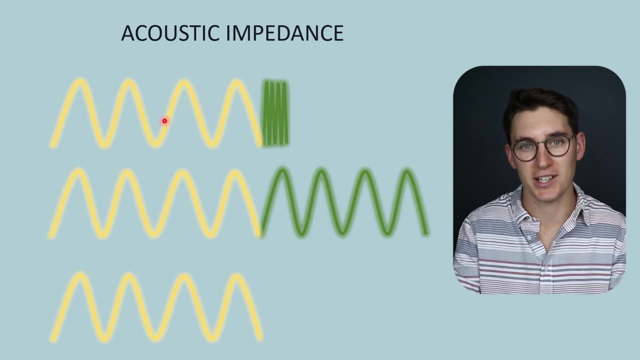 Now, if the acoustic impedance value of our tissue is high, it says that that tissue is stiff, it is resistant to compression. now imagine this as a spring here and we were to pulse a wave through that spring and that wave was to come into contact with a tightly packed spring. that wasn't. 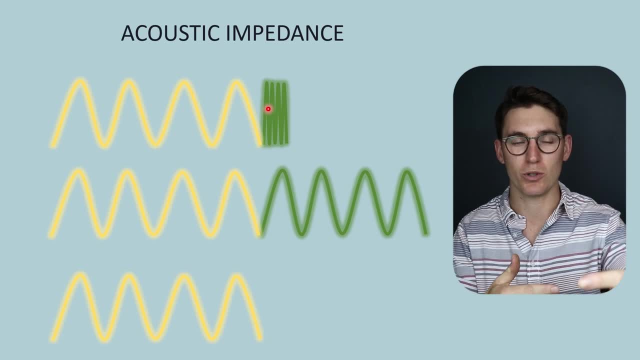 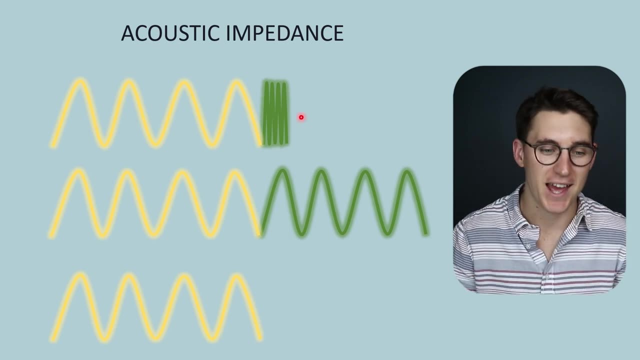 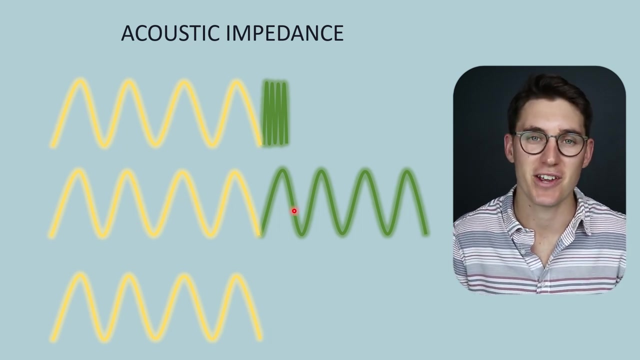 very compressible. it's much like this spring being attached to a wall and if you were to pulse it back, you can see how most of that energy will bounce back, be reflected as a pulse echo heading back towards where that wave came from. now, if we were to connect two springs that had very similar acoustic, 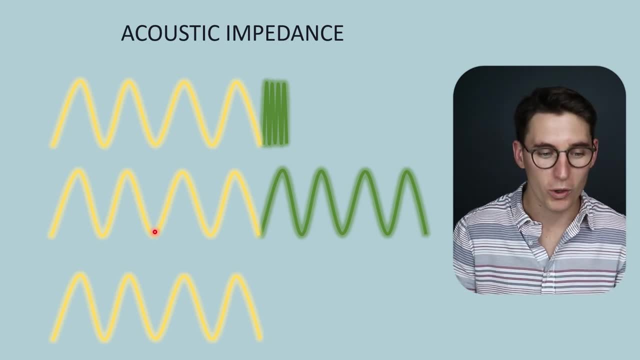 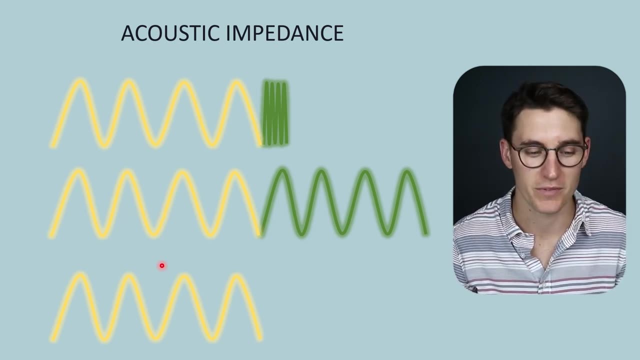 impedance values, we can see how that wave that we generate would most likely carry on as a wave as it heads to that second spring. there's very little reflection or echo. now, if we were to have a spring that wasn't connected to anything, it was connected to a tissue that was highly compressible, had a very 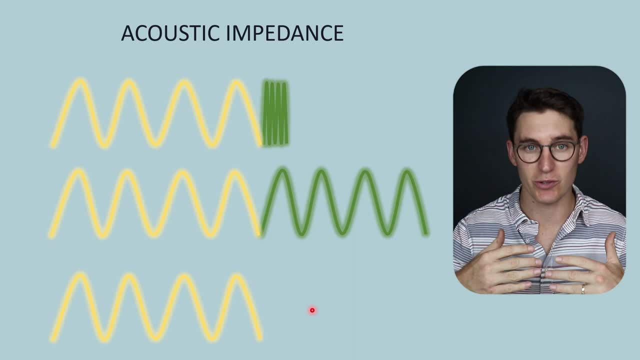 low acoustic impedance value, we can see that the energy reaching the end of the spring will have nothing to transfer its energy onto and that energy will then come back as those units in the medium rare effect come back to their resting place and that energy will then be transferred.